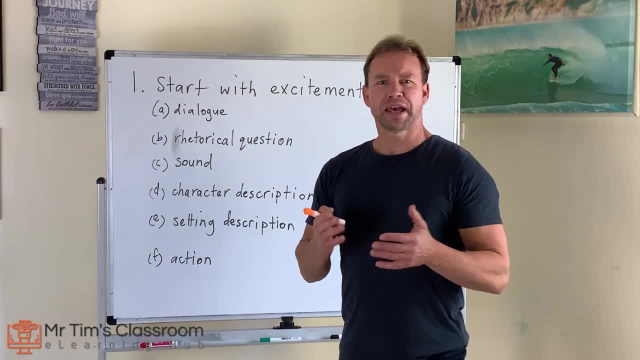 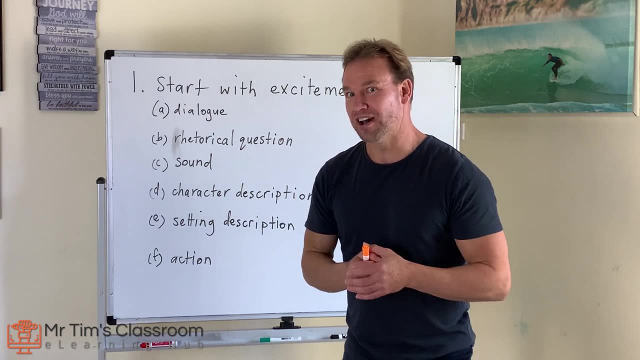 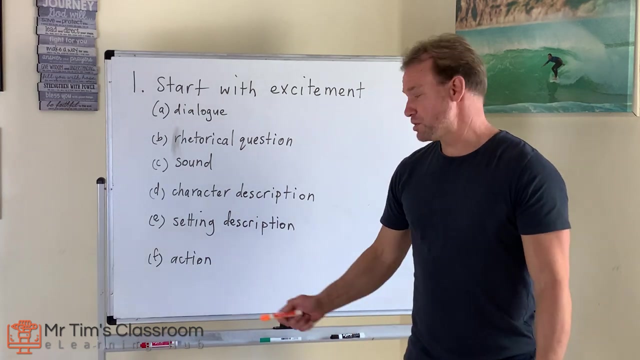 character. Maybe you could say something like: Max the Builder was a big, burly character with a nice moustache and a glint in his eye. Great way to start. You could describe the setting. Or probably one of my favourites is, you could start with some action. So, kids, that's my first tip: Avoid once. 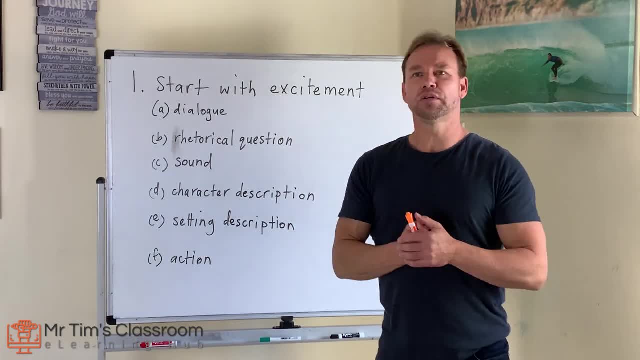 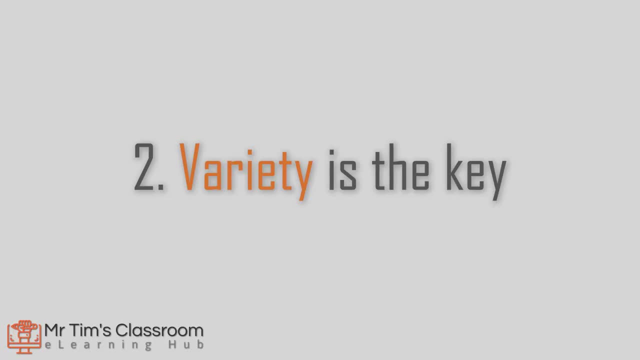 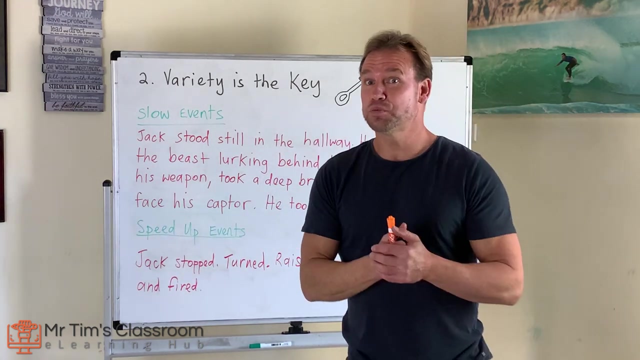 upon a time, one sunny day many years ago on a cold winter's morning, Doesn't really make the reader want to read on. That's tip number one. Tip number two: Variety. Variety is the key, Not only kids should we use a variety of sentence structure: Simple, compound, complex. 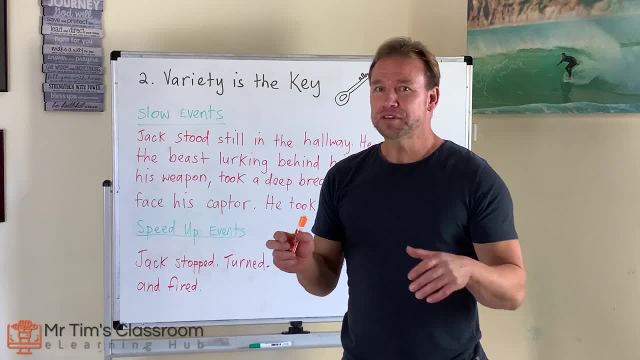 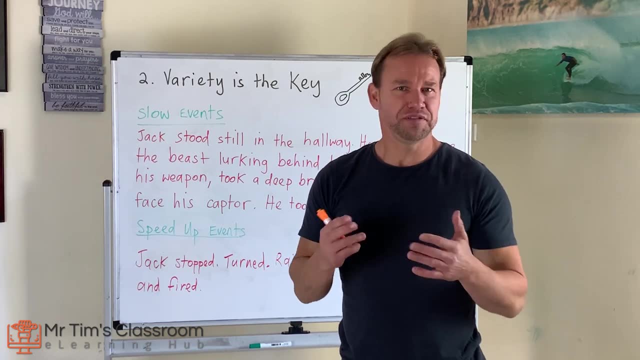 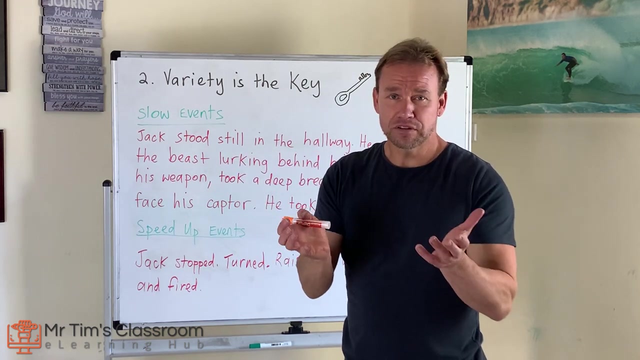 We should use a variety of vocabulary, right, Because this really helps to keep the reader engaged, And what you want to do is you want to make sure that it's not difficult to read. You want the reader to be able to flow over the words and get the meaning, get the characters, get the plot without too much effort, right? 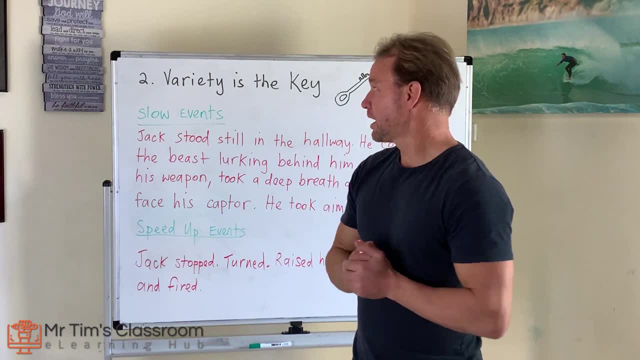 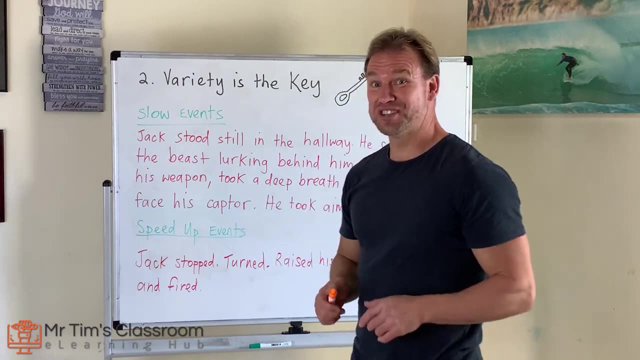 That's why using variety is really important. Now we can actually slow events down, and we can speed them up too with our sentence structure. Let's have a look at this example. So let's have a look at this Slowing events. 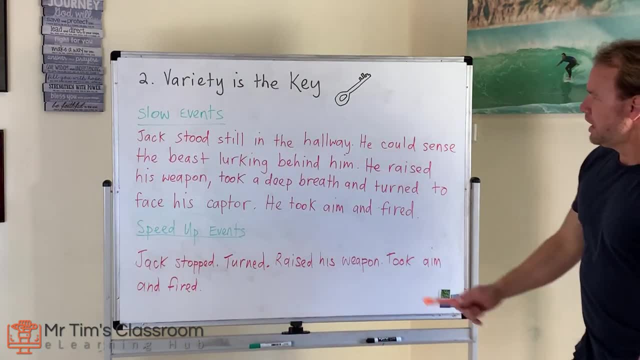 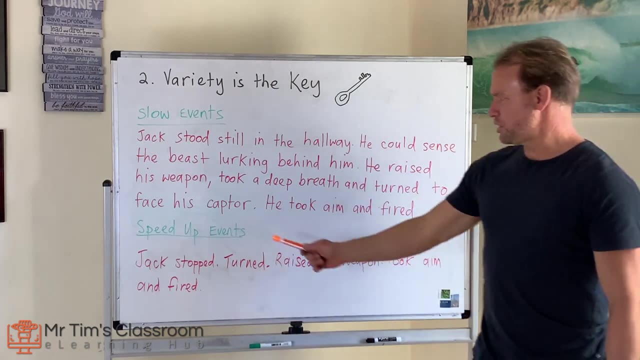 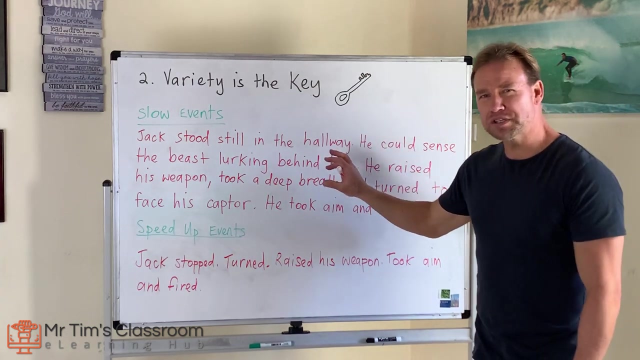 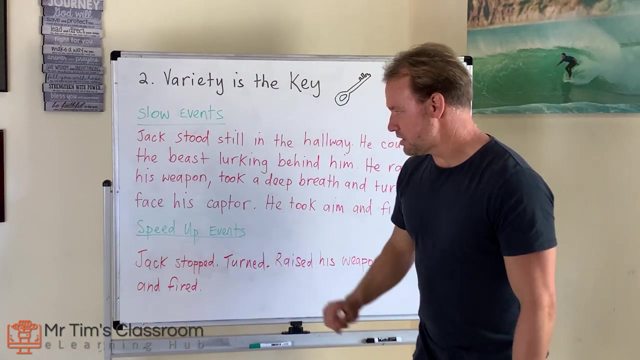 So Jack stood still in the hallway. He could sense the beast lurking behind him. He raised his weapon, took a deep breath and turned to face his captor. He took aim and fired. Okay, that's quite slow, isn't it? It really paints the picture in a lot slower way than if we did it like this. 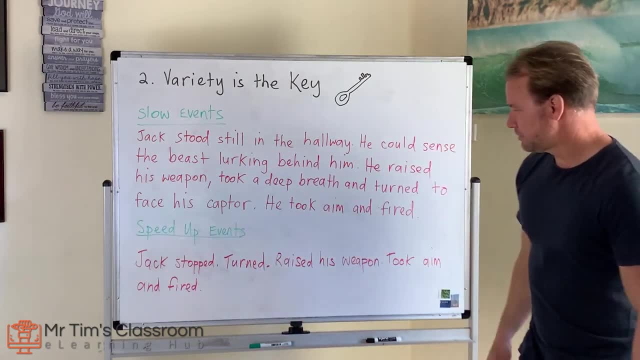 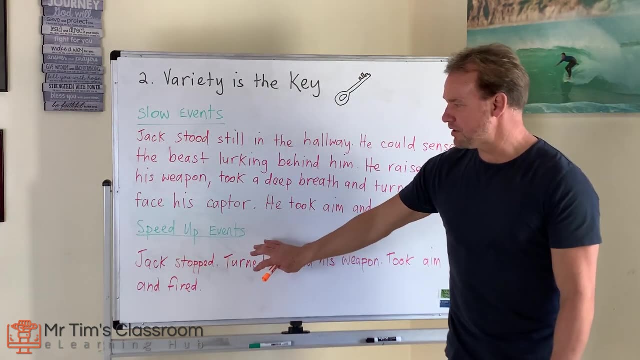 This is really speeding it up. Look, Jack stopped, turned, raised his weapon, took aim and fired right. So you can see, you can get a feeling that there's more urgency in the second part, in the speed it up events, than there is here. 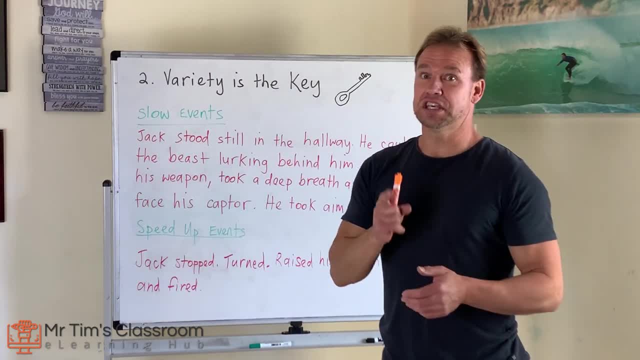 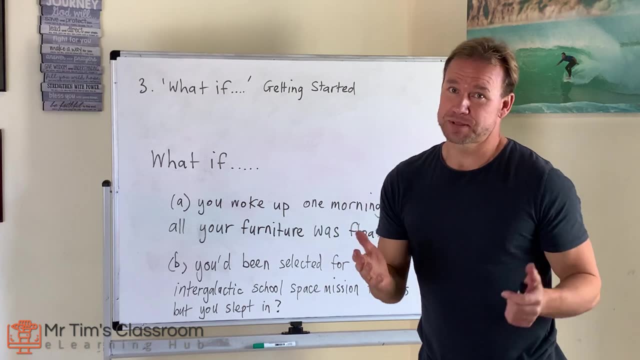 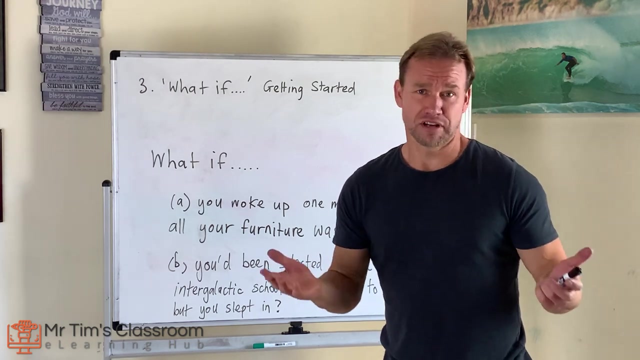 So number two: kids. Variety is the key. Okay, kids. time for tip number three. You know what? Getting started is sometimes the hardest part. I remember when I was a kid I really found it hard to get started and I used to write the same story basically over and over again. 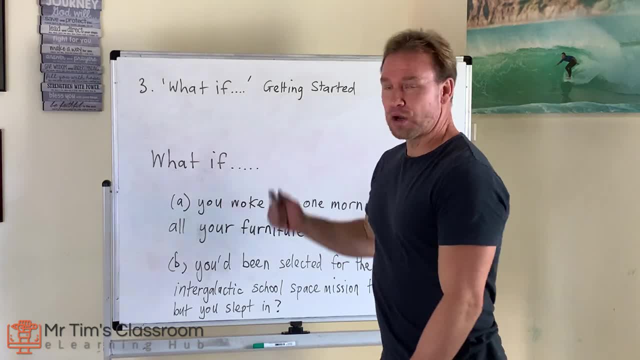 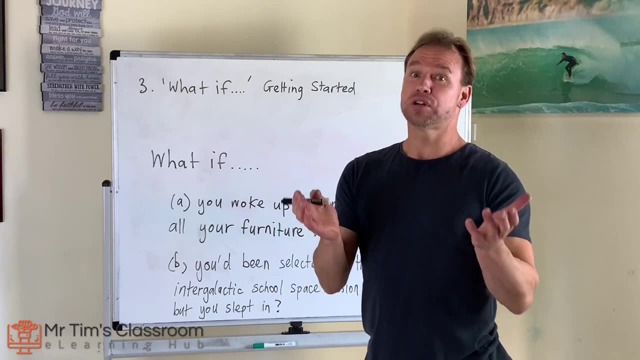 So what can we do? We can ask a what if question, right? A what if question is just a short question that basically summarizes the whole plot of a story. right, Let's have a look at this example. So imagine: 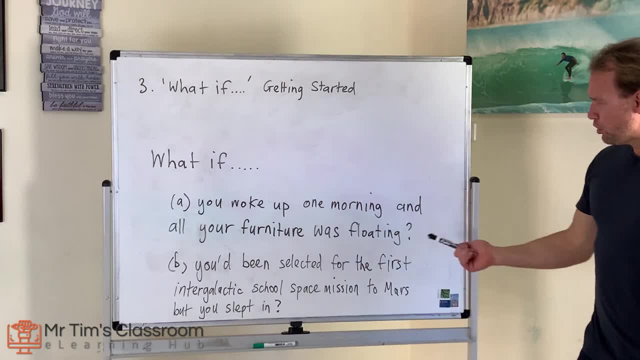 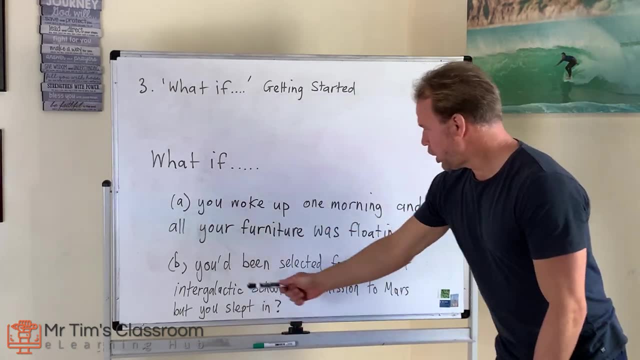 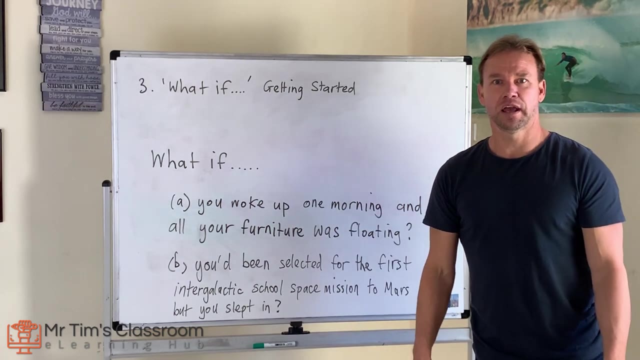 What if you woke up one morning and all your furniture was floating? Hmm, that'd be very weird, wouldn't it? Or this one: What if you'd been selected for the first intergalactic school space mission to Mars, but you slept in? 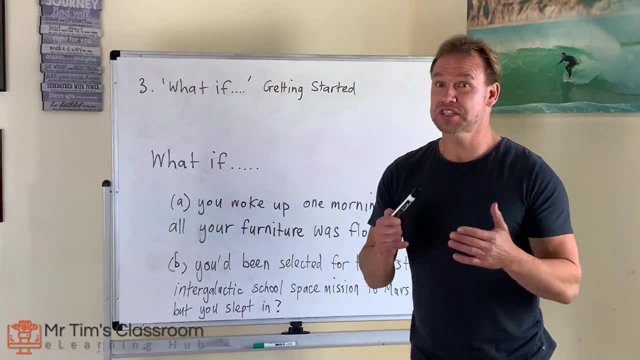 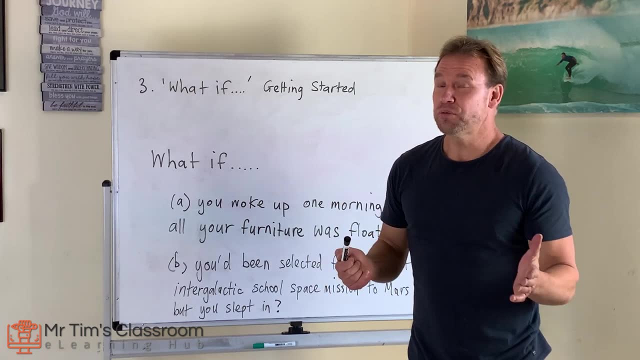 What if? question is a really good way, guys, just to stimulate your imagination and at least to get something down on paper, Because you know what You need: a map to get where you want to go right. So what if questions is tip number three? 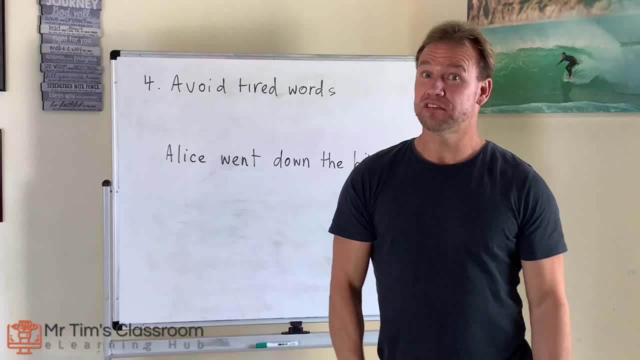 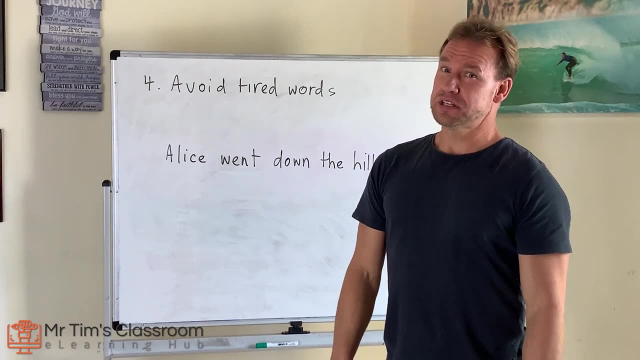 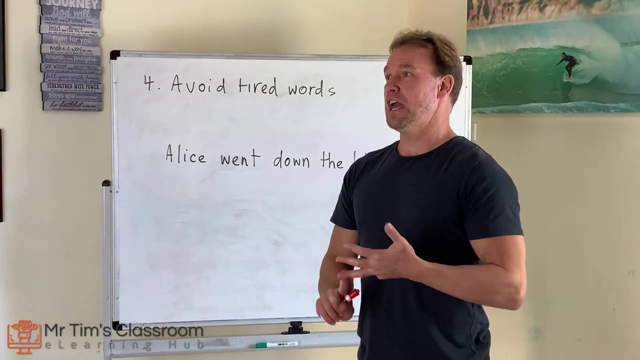 Tip number four, And I really think this might be the most important one: Avoid tired words. Do you know how annoyed teachers get when they see words like nice and big and small and thing and stuff and got and said and went and good and bad? 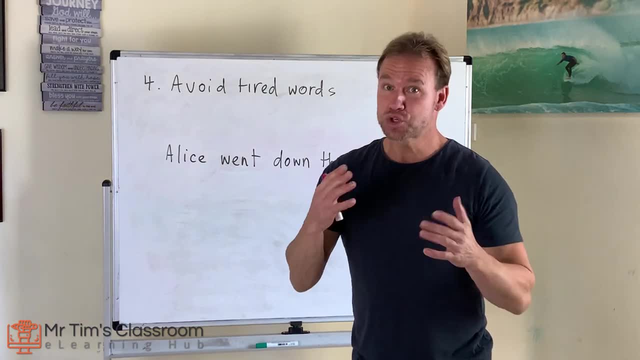 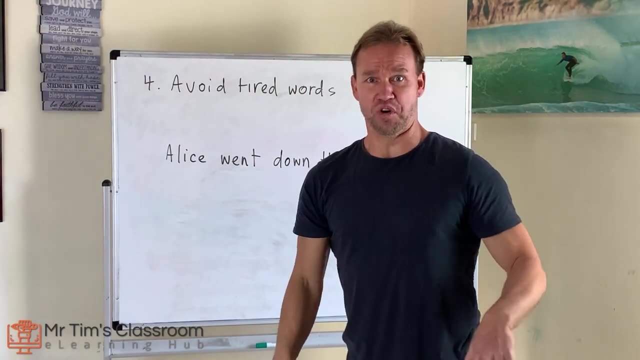 Try to avoid those words, kids. I'm sure you've all got a thesaurus right. Thesaurus is not some kind of dinosaur like a stegosaurus. Thesaurus is a kind of book that you use that you can get synonyms. 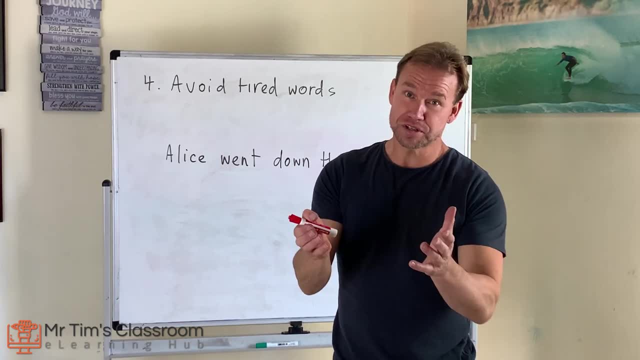 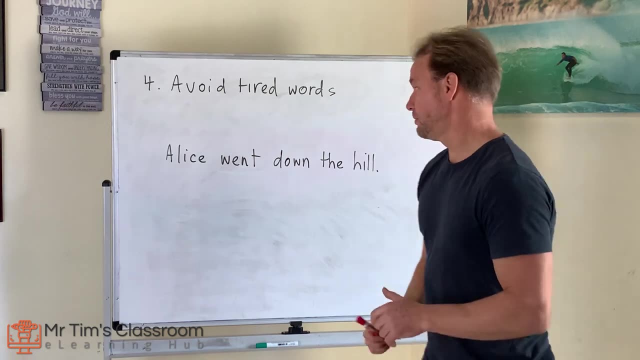 So if you want a word for big, you go into the thesaurus, you go to big and there will be lots and lots of alternative words that you can use. Let's have a look at this example. right, Alice went down the hill. 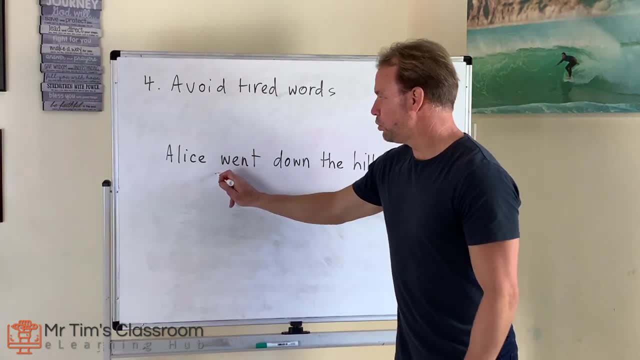 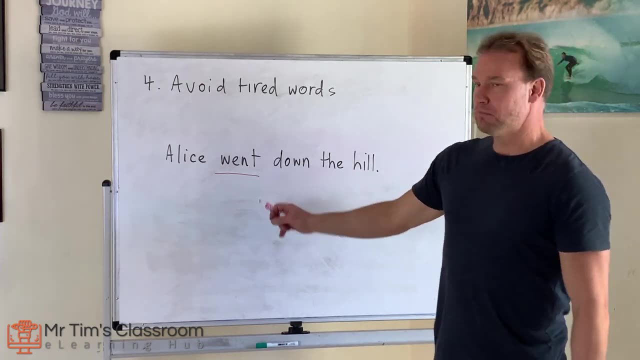 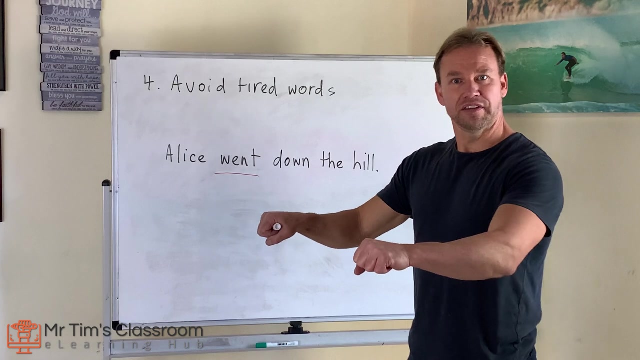 Okay, The boring word there is went. How many different ways could Alice go down the hill? She could march down the hill, She could skip down the hill. She could stroll down the hill. She could ride down the hill, She could skate down the hill. 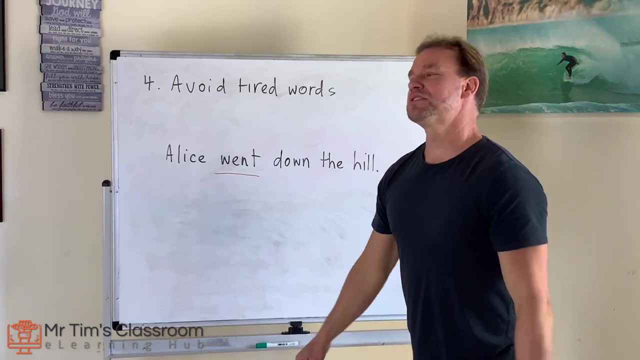 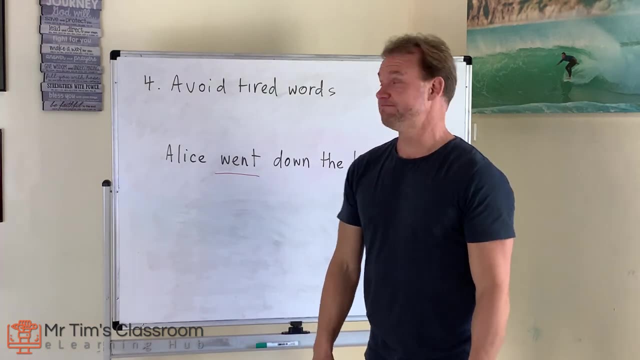 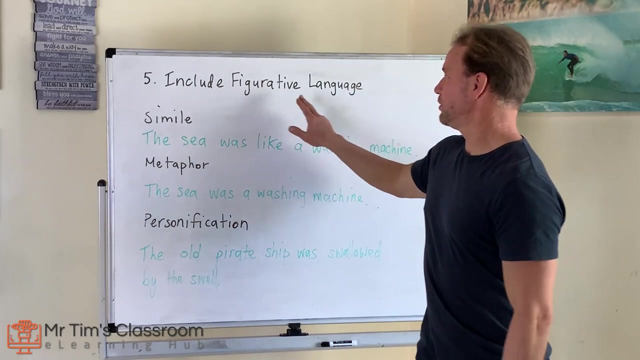 She could roll down the hill, She could stagger down the hill. So many alternatives. Try to avoid went. You don't really need it. That's tip number four. Okay, kids. Tip number five Include figurative language. Have you heard of figurative language before? 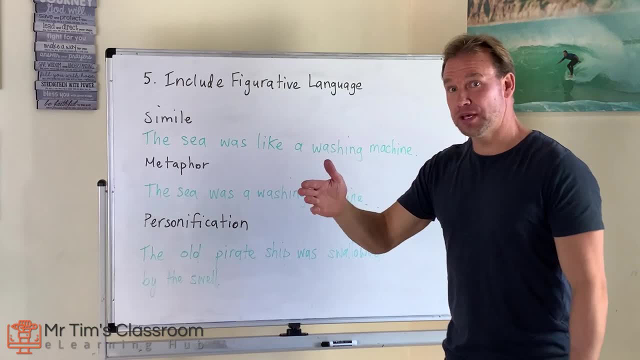 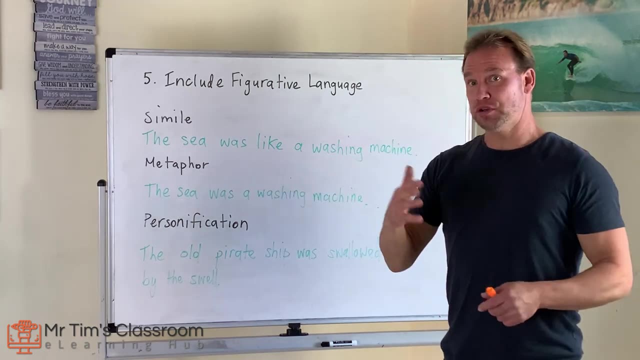 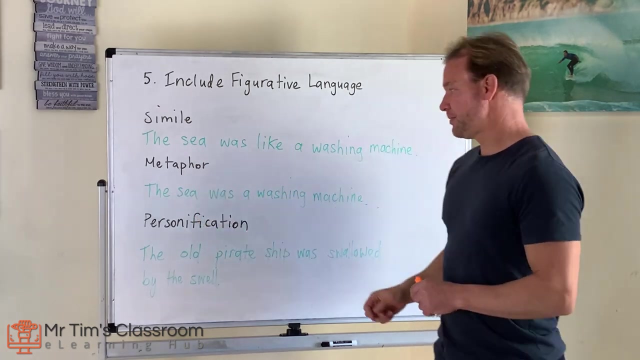 Techniques like simile is when you compare one thing to another. using like a or as a Metaphor is when you compare, but we don't worry about the like or, as We just say something. We just say something is something else or was something else. 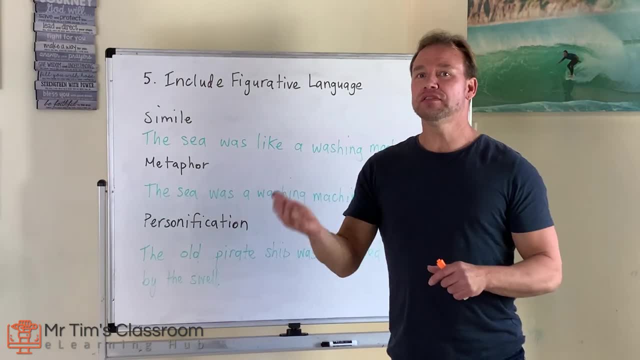 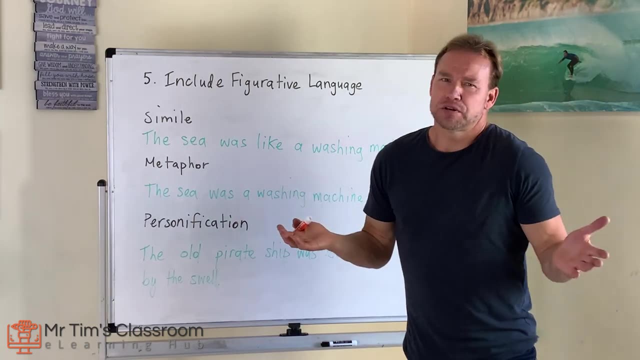 Personification is when you give a non-living thing or a non-human thing a human quality. Let's imagine that we're writing a story about I don't know some pirates out at sea. Okay, And we want to describe the sea. 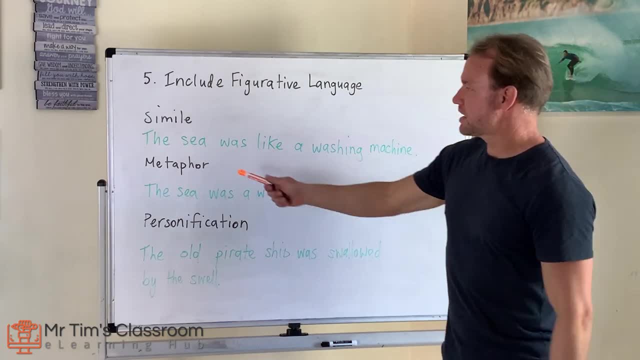 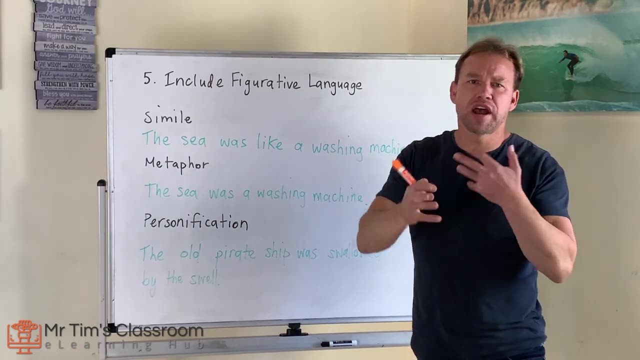 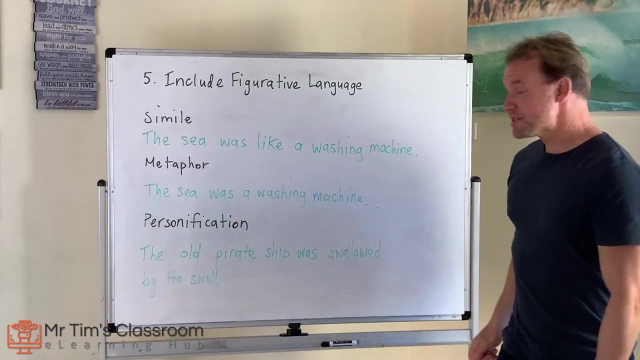 Maybe the sea was really wild and rough. So we can say the sea was like a washing machine, Churning White water, moving around, Dangerous. Now, if we want to turn that into a metaphor, we can say: the sea was a washing machine. 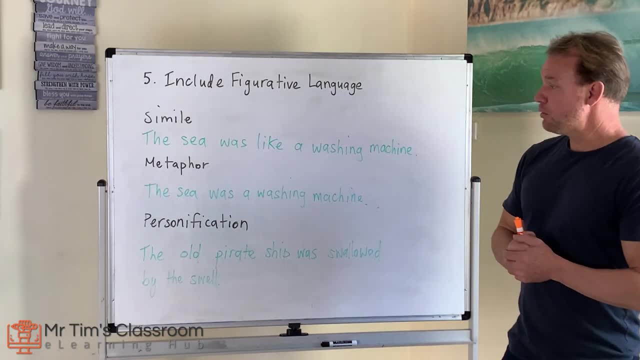 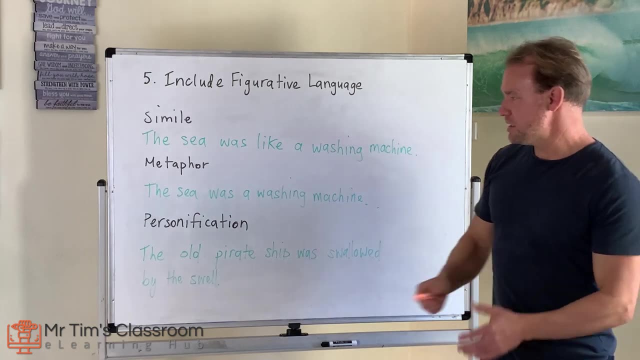 We get rid of the like a. Okay, Now, if we want to play around with personification, we want to bring the sea to life. We could say something like this. We could say: the old pirate ship was swallowed up by the swell. 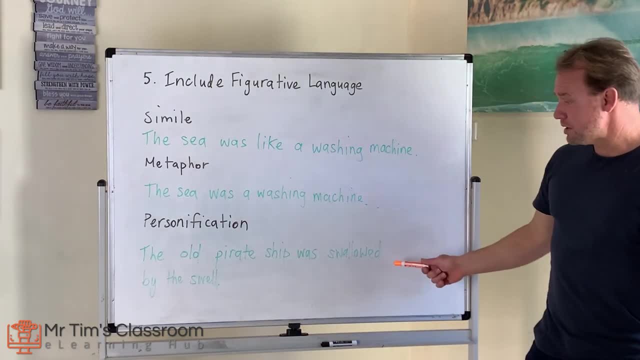 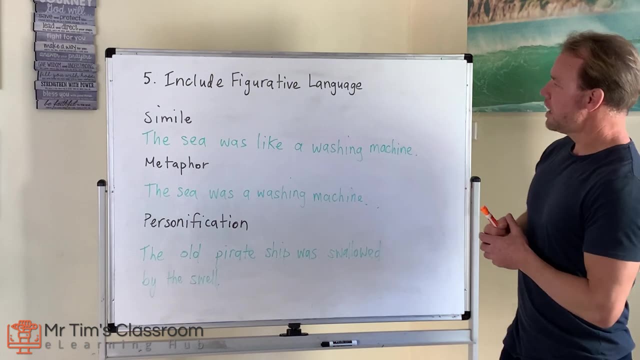 So the swell is like the big waves. So swallowed is not a characteristic that a sea has, That a sea can have. Right, People can swallow. So kids play with figurative language. That's tip number five. All right, kids. 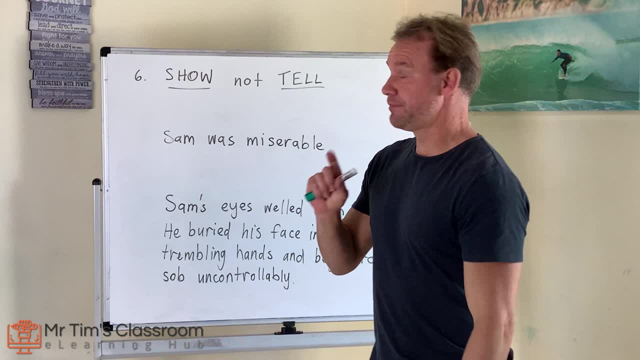 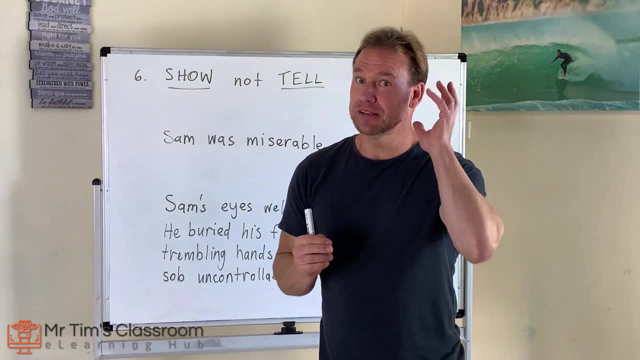 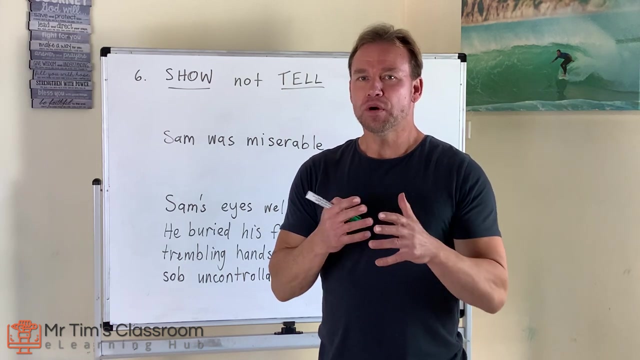 Tip number six: I love this one: Show, not tell. You know, really great writers are able to paint a very clear picture in the reader's mind. This is done with language. So if you always tell the reader the emotion of the character, they don't need to do any work. 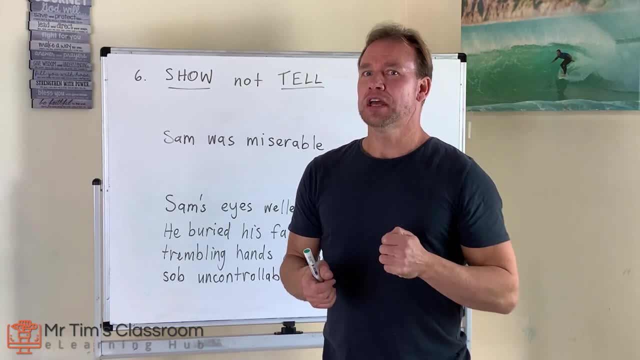 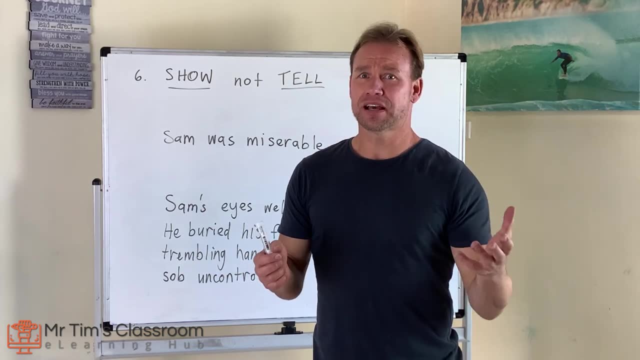 They don't need to visualize anything in their mind. And is that going to be a successful story? Is that how we're going to paint a picture, by telling the reader exactly what's going on all the time, Or do we want to leave it to the imagination of the reader? 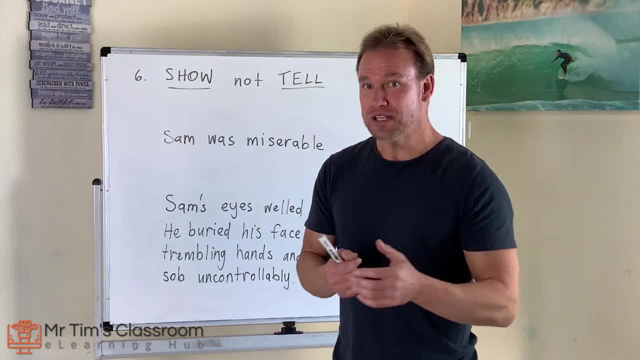 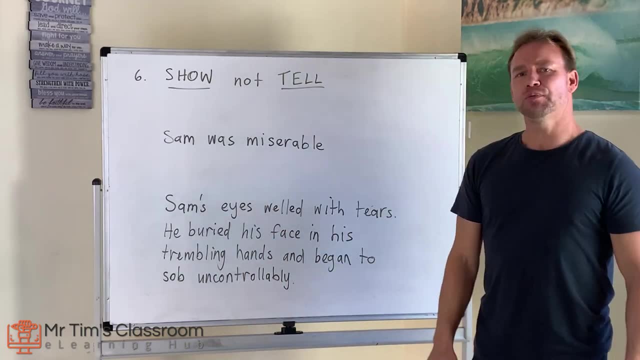 Of course that's what we want to do, right, That's how we engage them and entertain them. So let's look at these couple of sentences. This one says: Sam was miserable. Now is that show or is that tell? 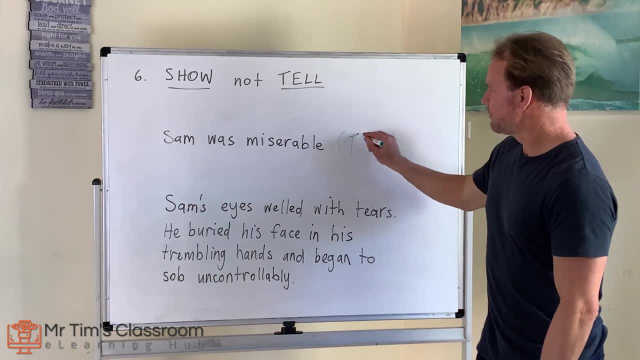 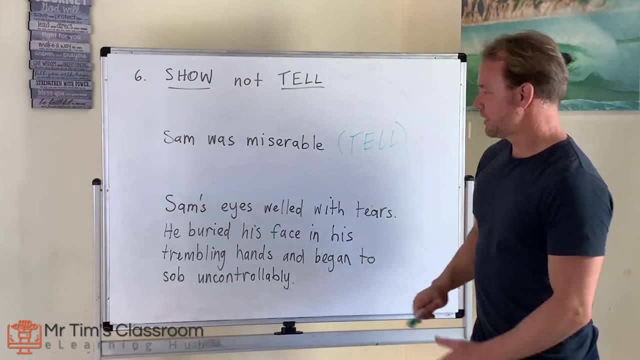 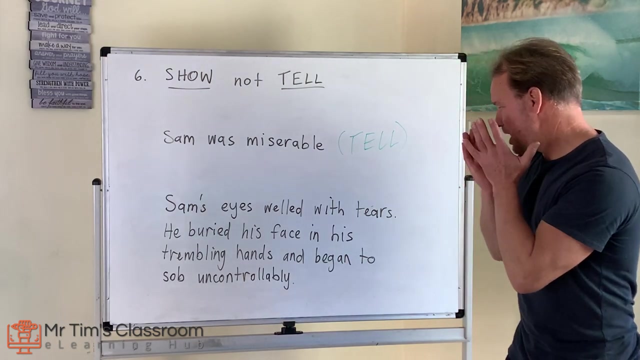 Of course that's tell. Okay, we're telling the reader how Sam feels. Let's have a look at this one. Sam's eyes welled with tears. He buried his face in his trembling hands and began to sob uncontrollably. 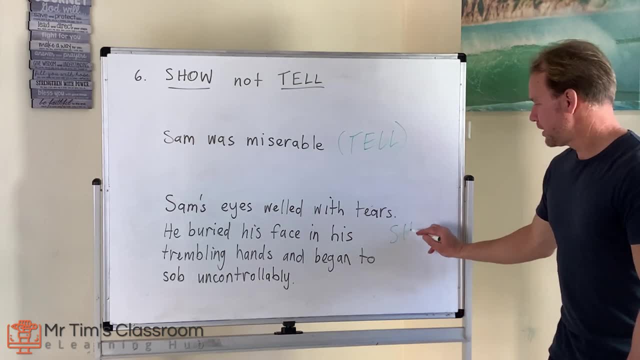 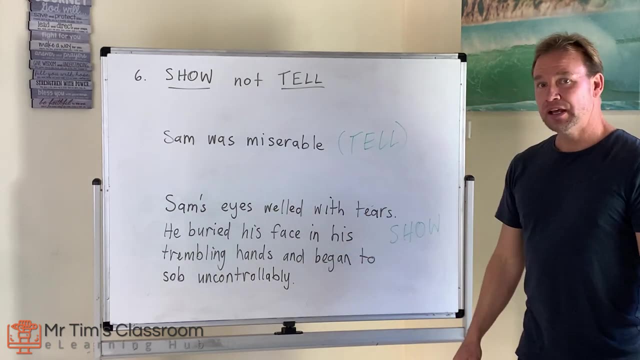 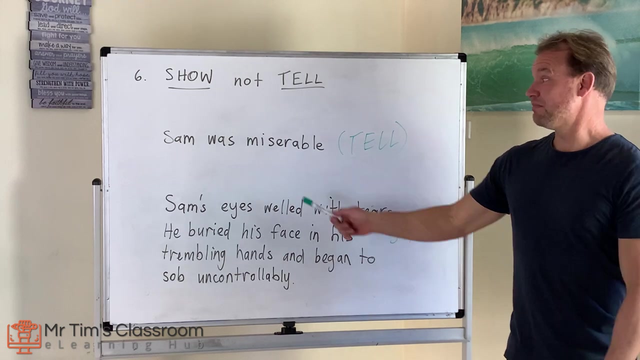 Obviously, kids, this is show, And you'll notice I didn't mention anything about being miserable or being sad, But you know because of the language that Sam is very, very unhappy. In fact he's miserable. So kids try to show, not tell. 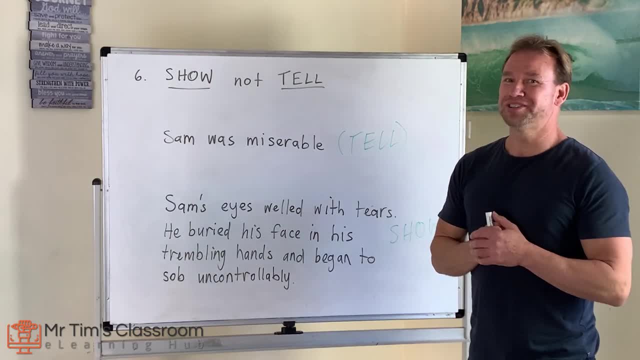 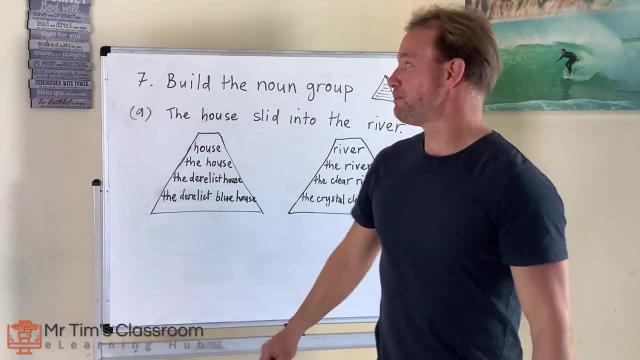 Doesn't mean all the time, But try, Try from time to time to show, not tell. Okay, That's number six. Alright, kids. tip number seven. This is our last one. Build the noun group. We want our sentences to sound interesting, right. 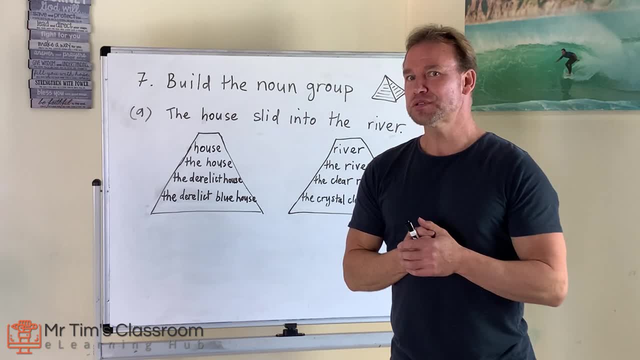 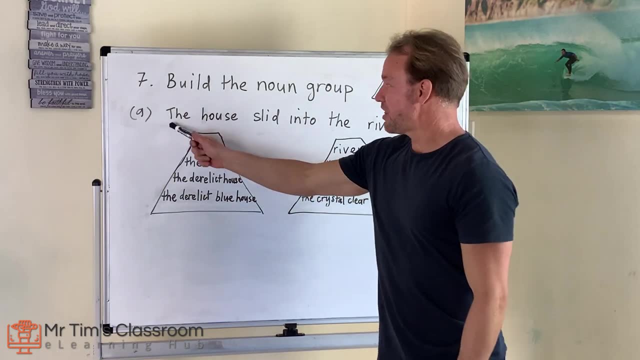 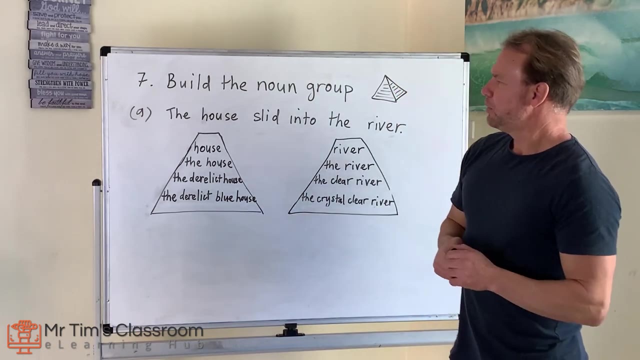 And descriptive, So we need to include: Do you know what they're called Adjectives? Let's have a look at this sentence together: Okay, The house slid into the river. Okay, It's alright, Nothing wrong with it, But we haven't got any descriptive words before house or before river. 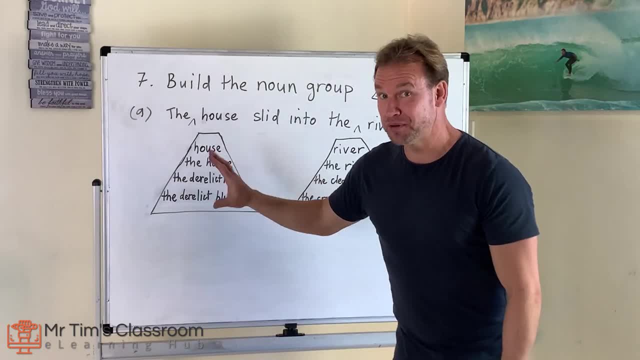 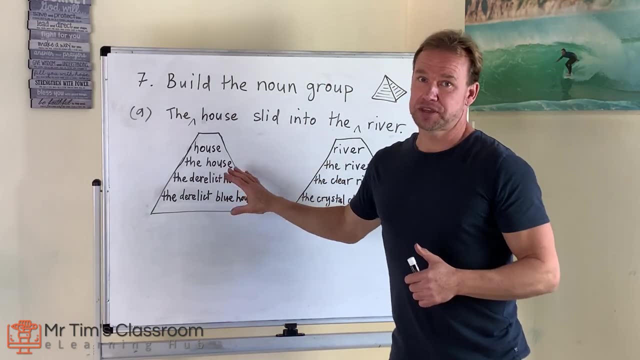 So what we can do is- I like to call these noun pyramids, Or you can call them noun volcanoes or whatever you want to call them, So you can actually physically do this at the beginning, But then after a while you do it up here.